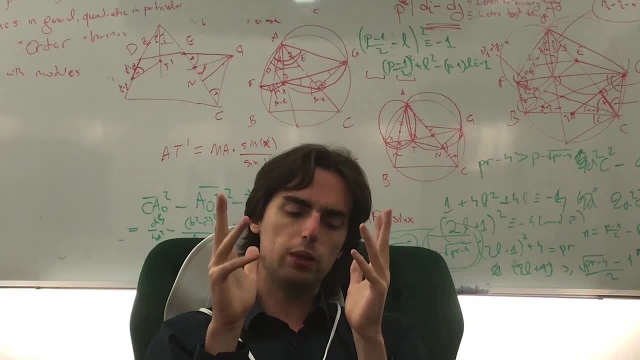 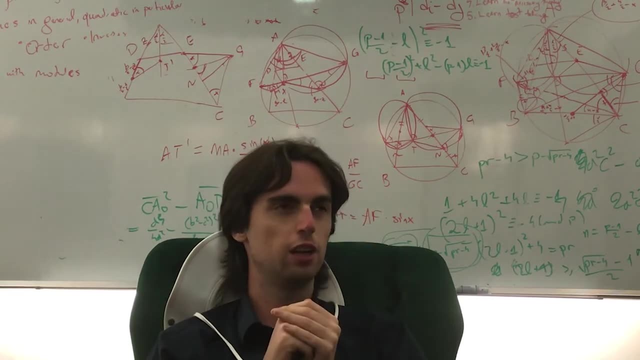 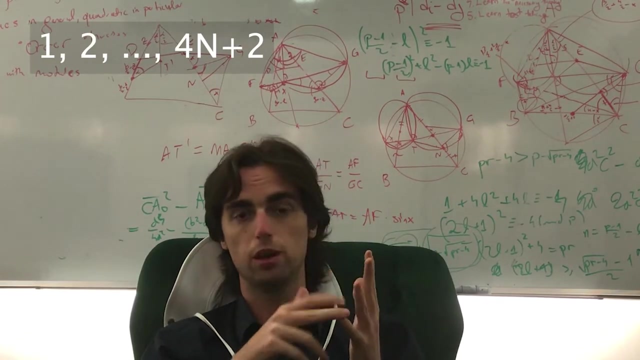 can actually prove this. But an example with invariance. we're actually looking at end states. Is there a problem where, say, n is a positive integer and you have numbers 1 through 4n plus 2 written on the blackboard? So you have 1, 2,, 3, 4,, all the way until 4 times n plus 2.. 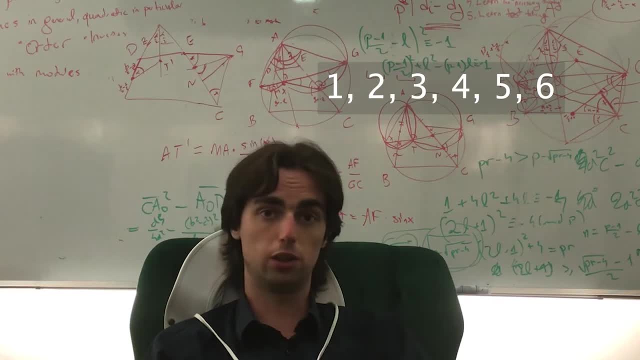 An example is: say you have numbers 1,, 2,, 3,, 4,, 5,, 6 written on the board And at every turn your friend takes 2 of these numbers and writes this absolute difference on the board. So it takes: 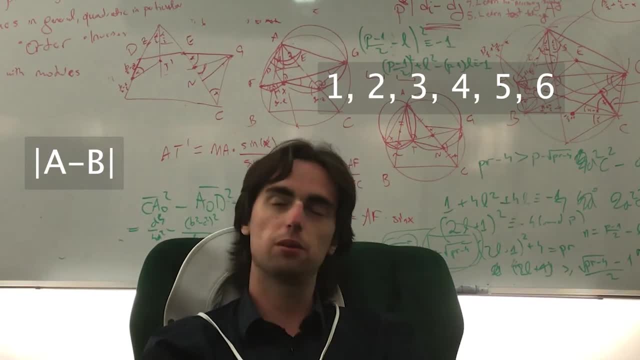 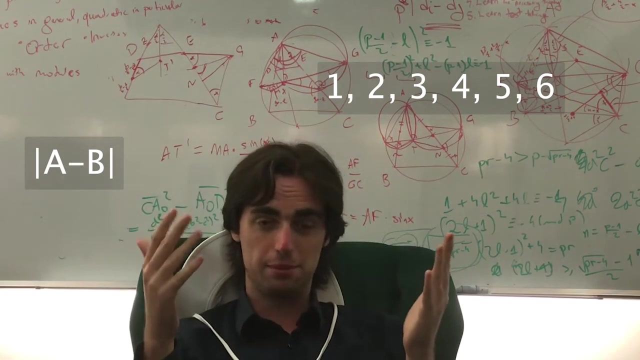 two numbers, deletes them and writes their absolute difference on the board. And the problem says: can a 0 be written on the board at the end? And the answer is: well, there's an invariance here happening. So what is something that? 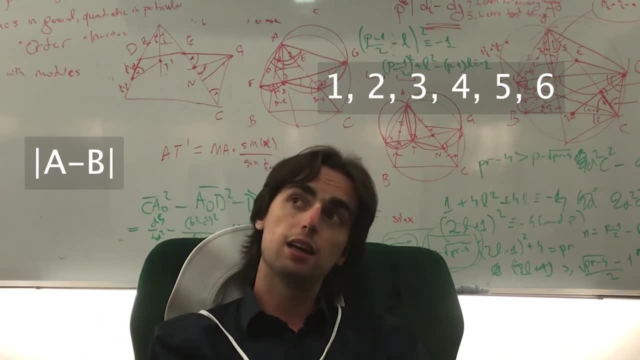 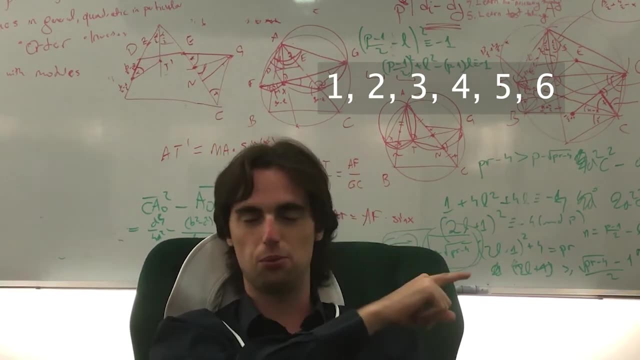 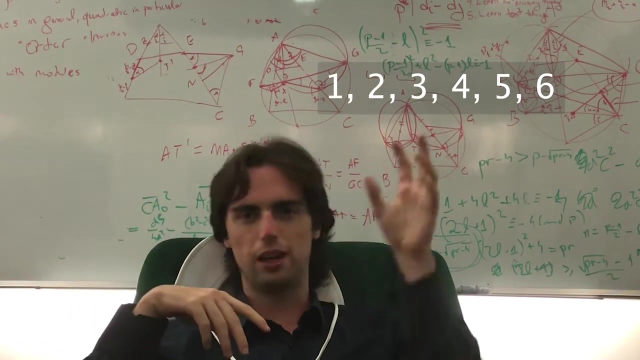 remains constant while you're writing a minus b. The thing that does remain constant here, say: if you write, if you take 2, if you have 1 and 2, you'll have 1.. If you have numbers 1,, 2,, 3,, 4,, 5, 6,, you take 6 and 4, you have a, 2, 2, 1, 3, and 5.. 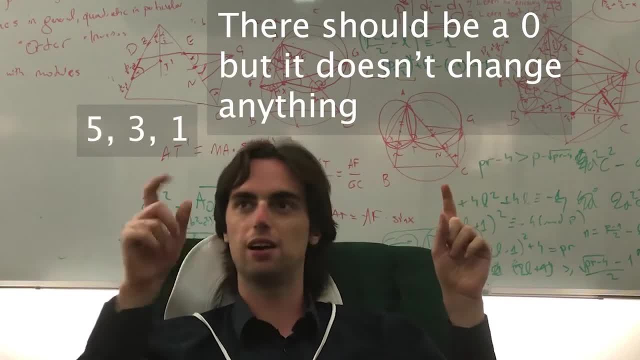 You take a 2 and 2,. you have a 1,, 3, and 5.. You take a 5, 3,, you have a 1, 2,, but something while you're doing this, so you can have a 1. at the end you can have a. 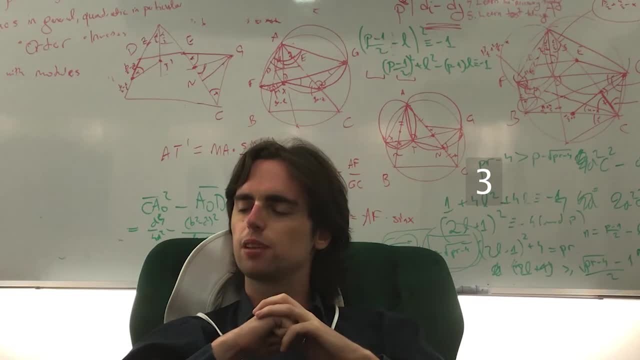 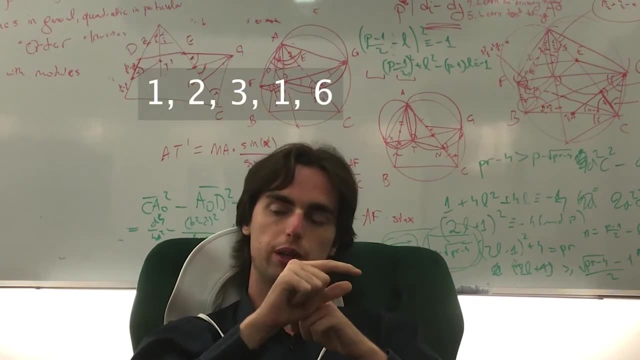 3. at the end And as you try out different transformations, you may find that, say, if you take 5, 4, you get 1,, 2, 3, you get 1,, 1, 1, you get 1,, so you have 1, 6,. 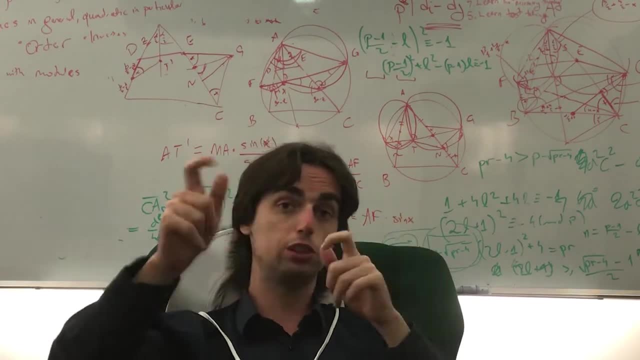 you can get 1,, 3, and 5 on the board And once you try different stuff out, you see that the only numbers you can get on the board are 1,, 3, and 5. If you try, say n. 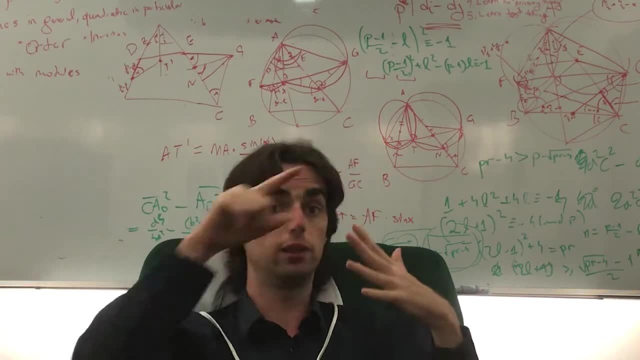 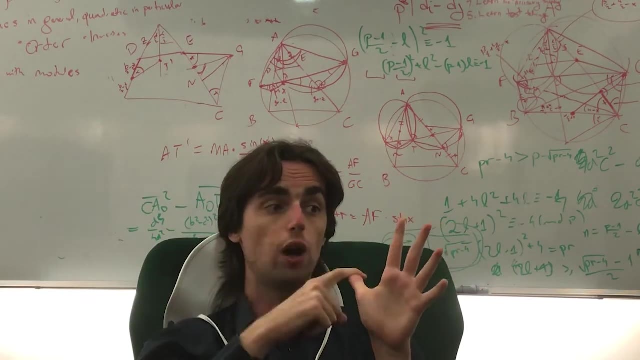 equals 2,. when you have numbers 1 through 10 written on the board, you'll see that what you have, you can get numbers 1,, 3,, 5,, 7, and 9.. I believe you can get all. 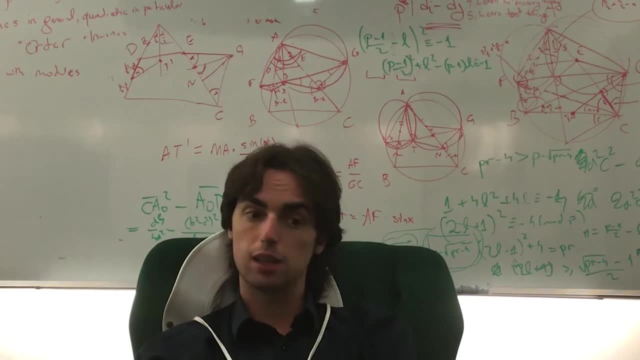 these numbers on the board at the end. And now the question is: why can't you get any of the evens? Now it's sort of hinting out: you're not going to be able to get 0 here at all, And the question is: why can't you get any of the evens? 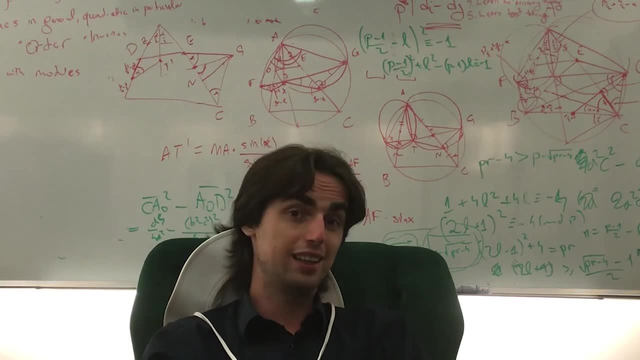 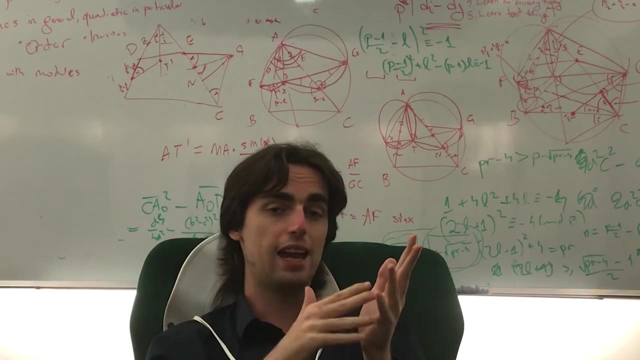 And what remains the same is- and this is a common invariant, and this is a common invariant, and this is a common invariant- that parity remains the same. If you delete the numbers a and b and you write a minus b in absolute values, what you're left with, say, if the sum of the 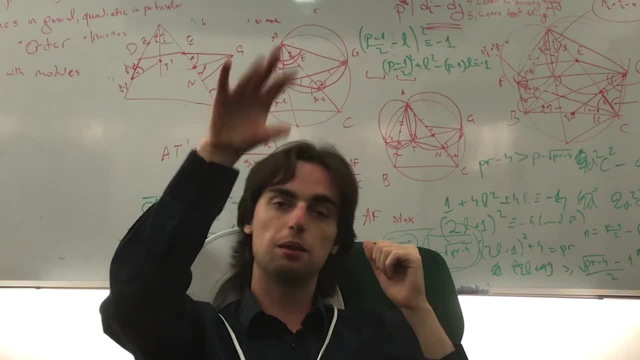 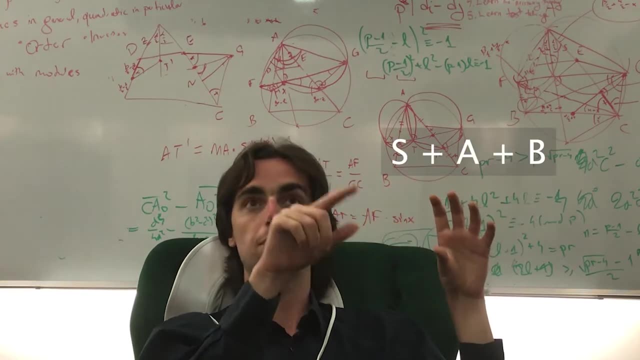 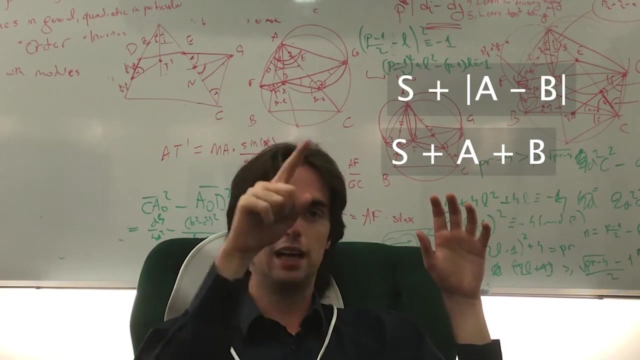 numbers before was of all the numbers aside from a and b. if it was s, then your total sum before you made the move was s plus a plus b. After you make the move, it's s plus a minus b in absolute value terms. Now, a minus b and a plus b have the same. 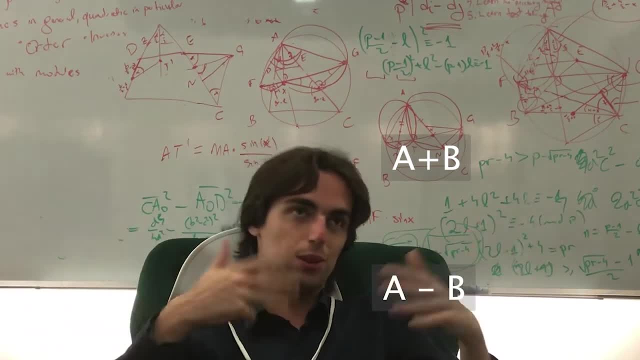 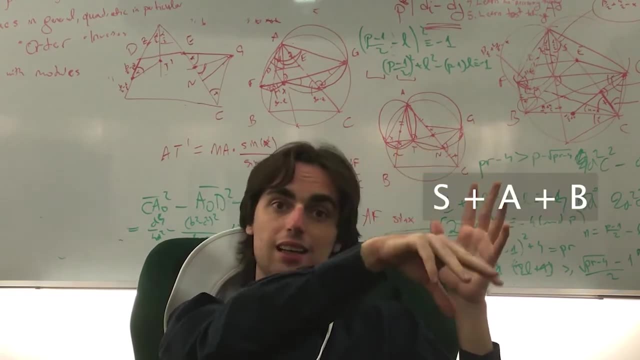 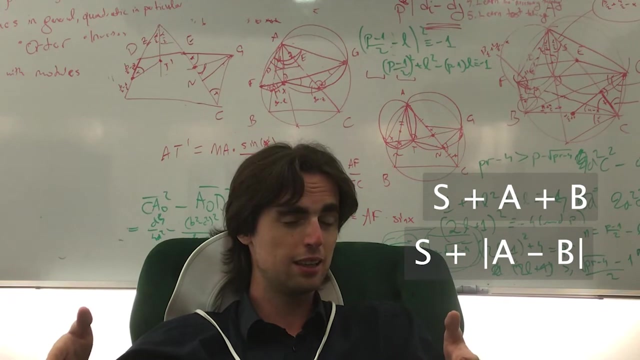 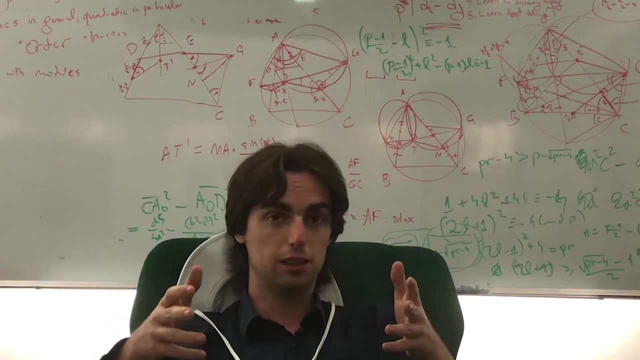 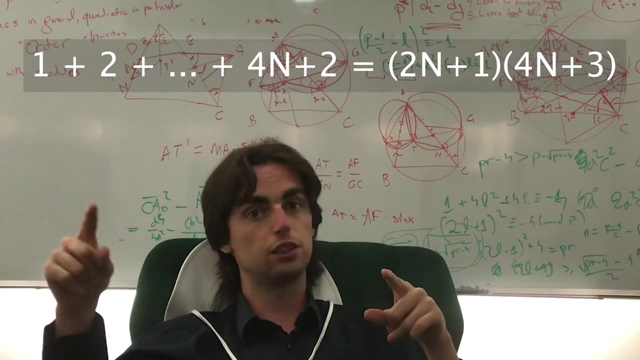 parity. You can test it out, you can prove this. they have the same parity. So s plus a plus b and s plus a minus b, in absolute value terms have the same parity. Now, given at the beginning that this whole sum is equal to n plus 2 over 4, n plus 2 over 2, so it's 2n plus 1 times 4n plus 3,. 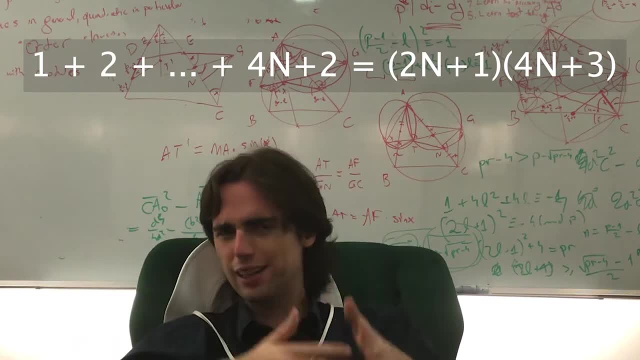 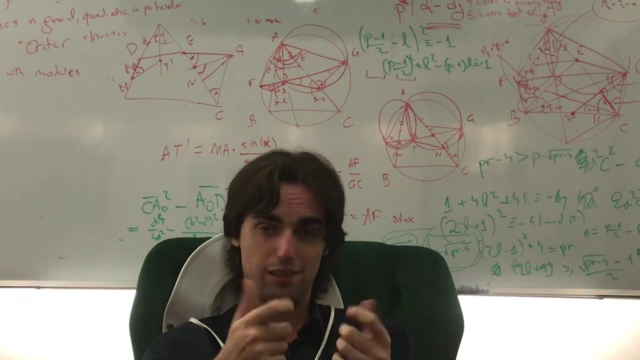 if I'm not mistaken, because that's the sum at the beginning and it's odd, that means at the end, because the parity remains the same. at the end, you'll also have an odd sum, which means an odd number. so that's why you can't have a. 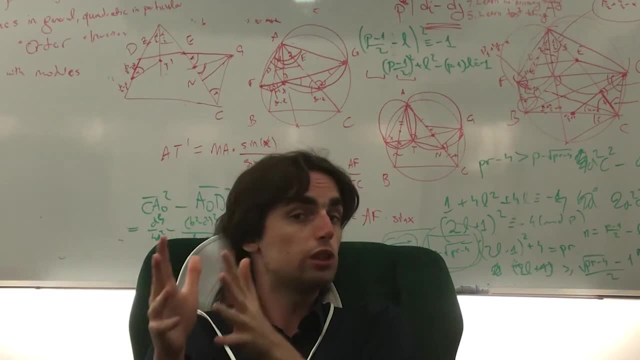 zero at the end. But this is an example of you looking at: okay, what's my end state, How can I, what are all my possible end states, How can I reach them? And then you're looking for different invariants. 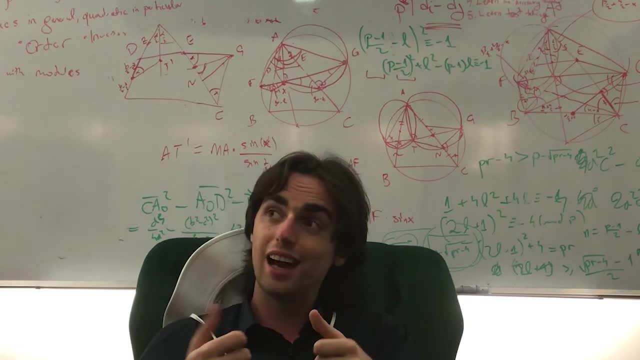 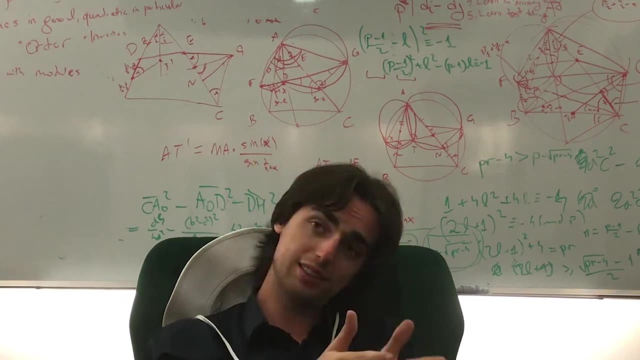 different things that don't change as the situation. the numbers written on the board change. So that's invariants in a nutshell, and how you practice this is with every technique. You have this little nugget I gave you and now go out. 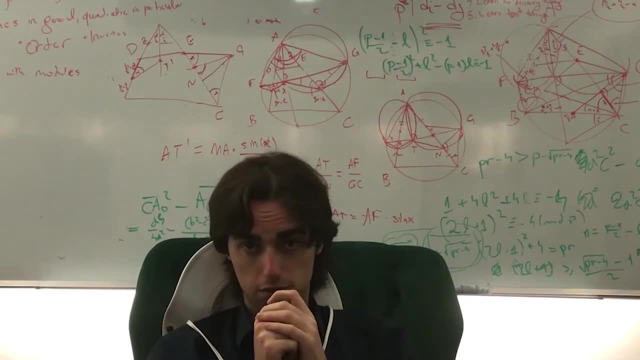 try to solve, maybe try to. if you haven't solved the three problems I've covered on invariants, please do. I might cover some more in the future and try to solve them. try to see if you come up with problems, if you see. 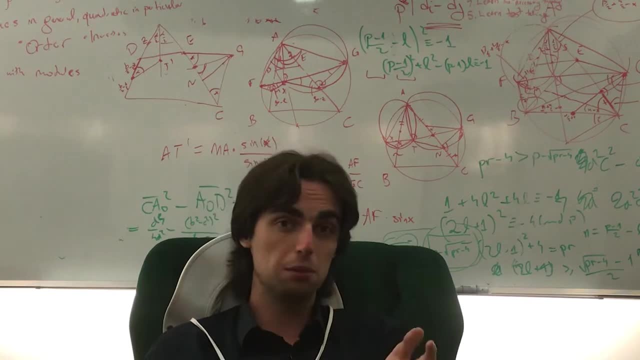 problems which use invariants. Try to see if you come across problems which, when you try to solve them, they have something that's changing and with that change, try to figure out: is there something that remains the same, Something I can control? 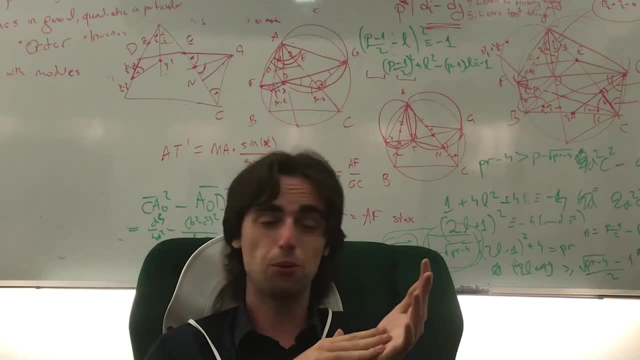 A good example of this is also, say, a game where you have 20 coins on a board, on a table, and two players take alternate turns and at each point you can remove one, two or three coins from the table. Who can win? This is basically a 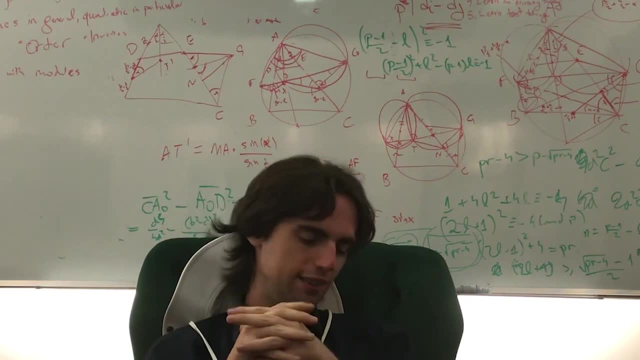 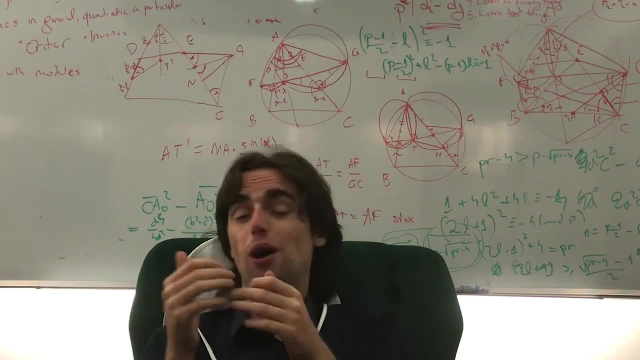 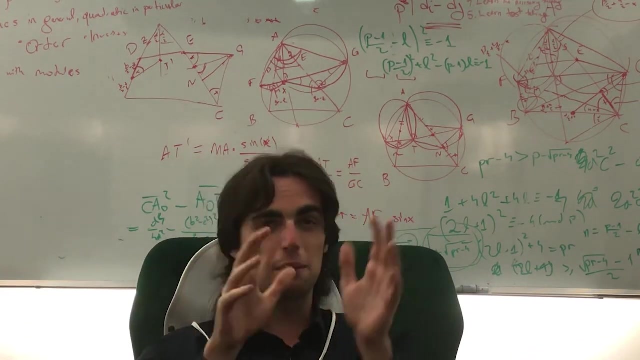 question, and this is a bit of a copying, maybe strategy sort of situation as well, but the potential invariant that one of the players can take advantage of is they can always have the sum decrease by four after their turn. So that's another cool invariant, and you come across these a. 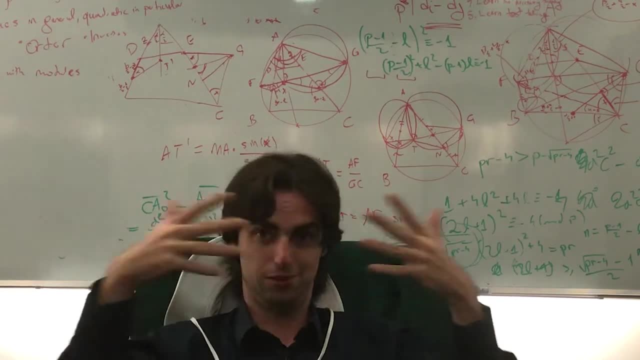 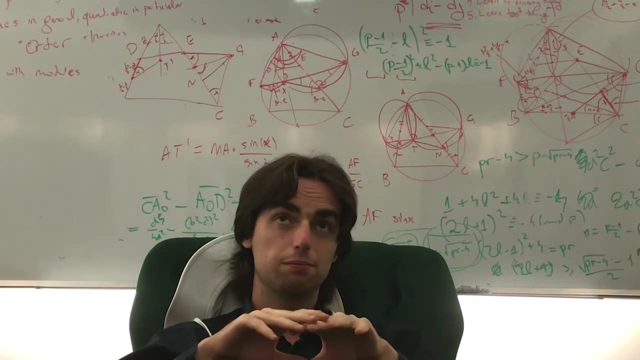 lot, but the thing is: solve problems and then you'll get better at this. And, most importantly here, that's the basic principle, and this is the basic principle. Now it gets a bit more complicated, but it gets a bit more. 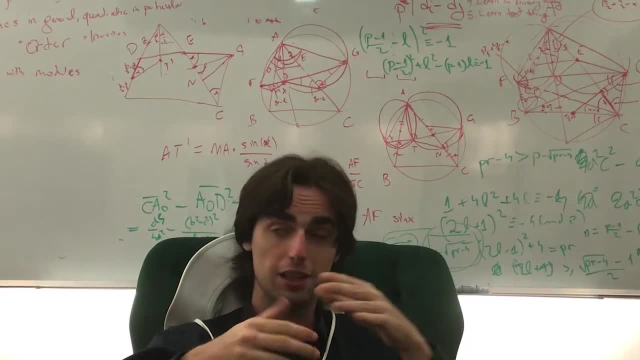 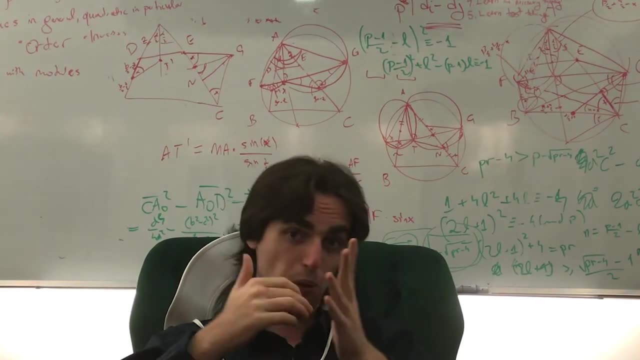 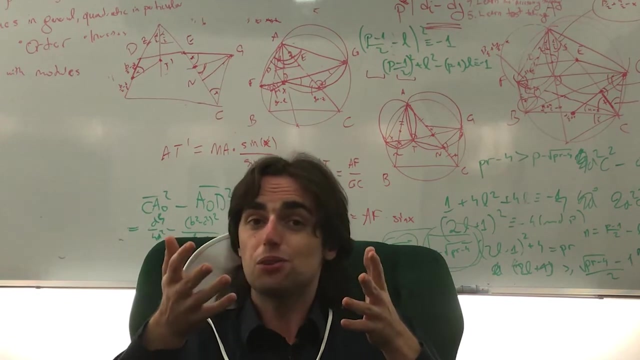 easy to apply. It can be applied to simple problems like the one I described here, or it can also be applied to very, very difficult problems. I can spoil a problem for you now, and the problem is from the 2021 IMO, A pretty difficult. 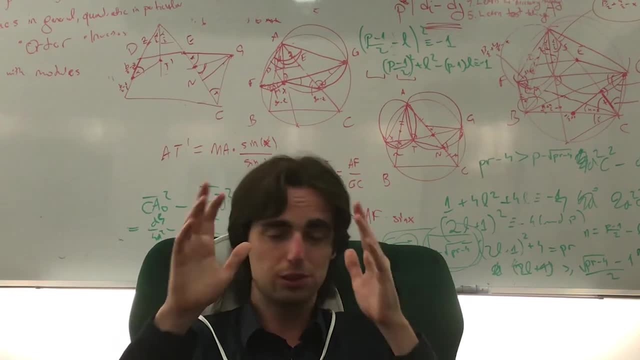 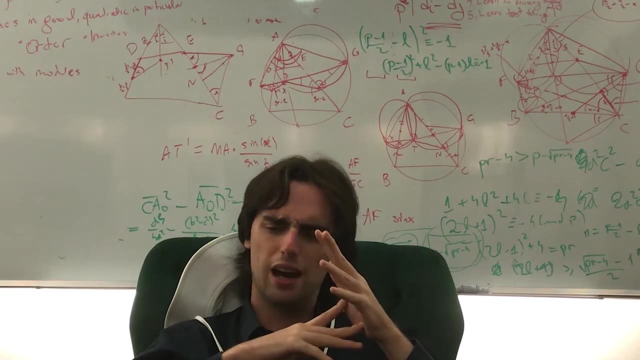 problem was just an invariance. It was one invariance that if you figured out you would solve the problem. I covered it on my channel. Or you have also an invariance. Even there was a problem that was a third or sixth at the IMO. 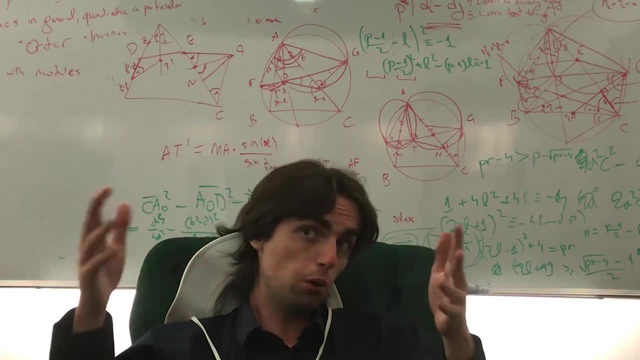 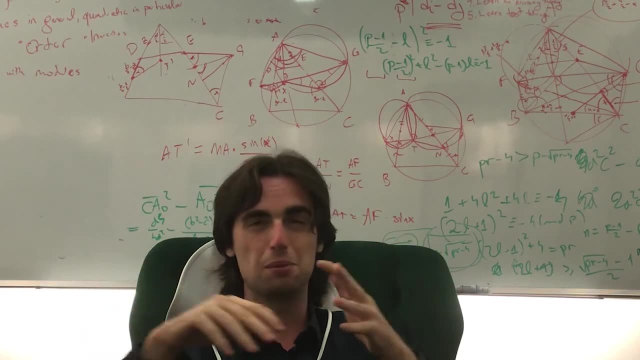 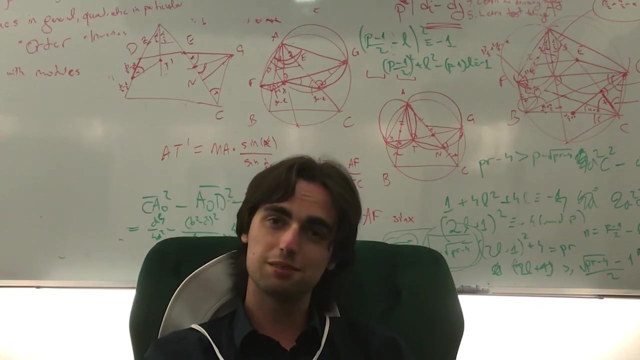 which used a bit of a complicated monovariance. It looked at something that changes in a controllable manner to come up with something and solve the problem. But this principle can be applied in many situations and now you're aware of it And, as always, thanks for problem solving.